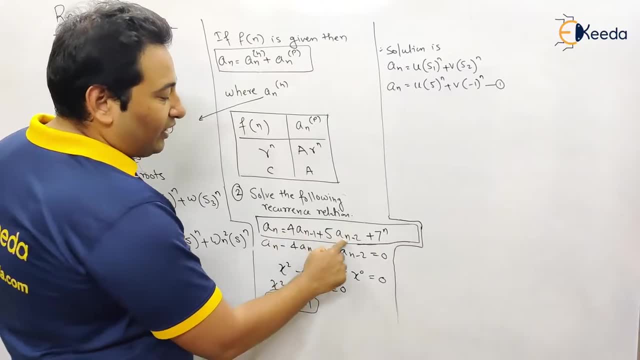 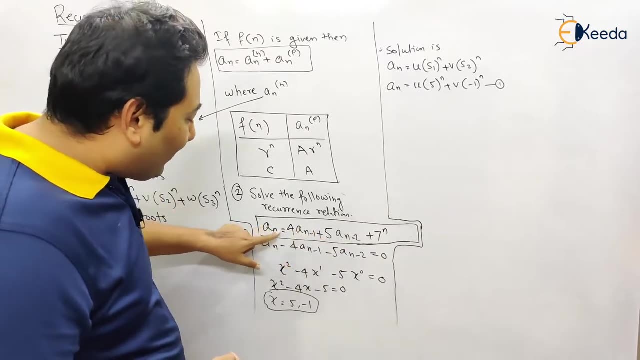 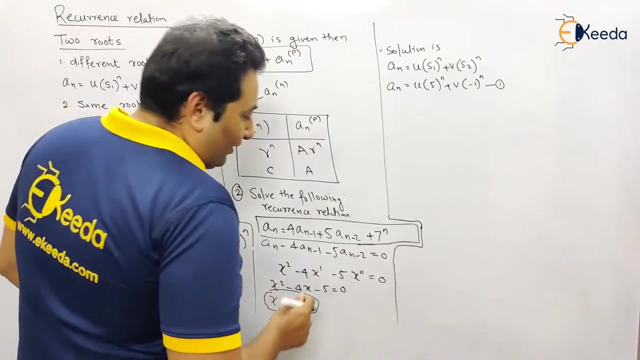 constant. see, whatever without a n is your f of n. a n, n minus 1, n minus 2. so whatever without a n, whatever you are left with is your f of n. so it can be of these two categories. So what is the first step? now, steps are similar. take these terms to left hand. 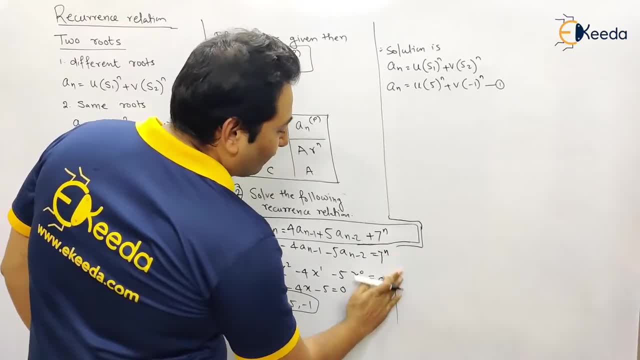 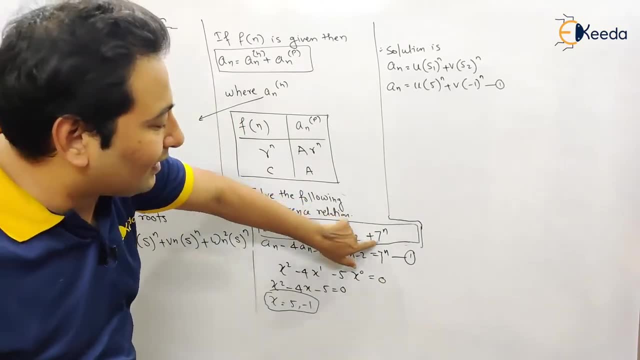 side, and here it will not be 0, here it will be 7 raised to n. so this is your equation number 1. so what I did? these two terms take to the left hand, left hand side, and 7 raised to n, and after that convert it into quadratic equation. 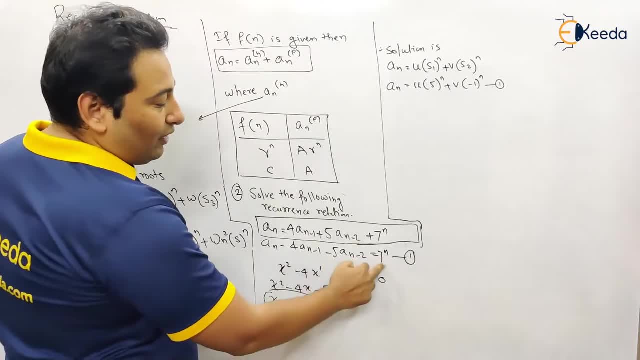 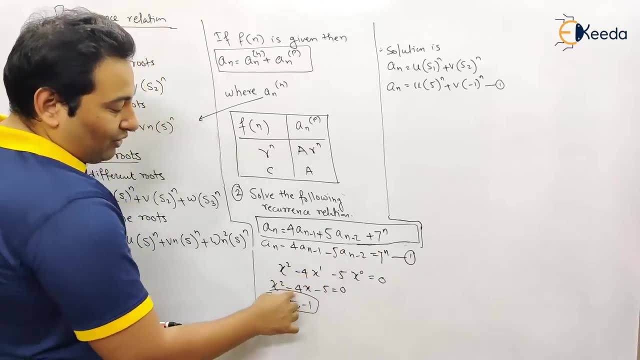 in terms of X and while writing down, we're going to take it as 0. we're not going to consider 7 raised to n, just we're going to take it as a 0, and the same procedure will get the values x equal to 5 and minus 1, and 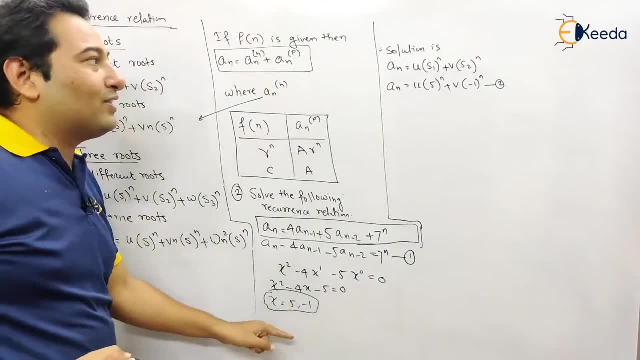 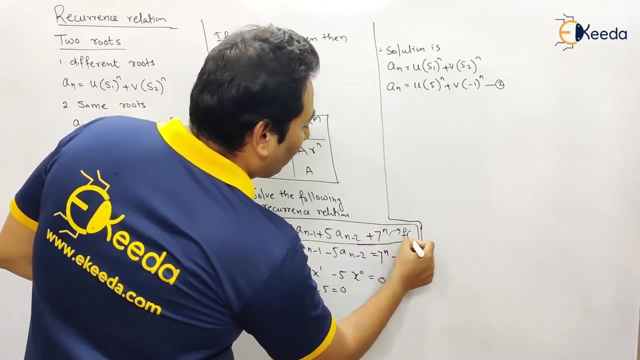 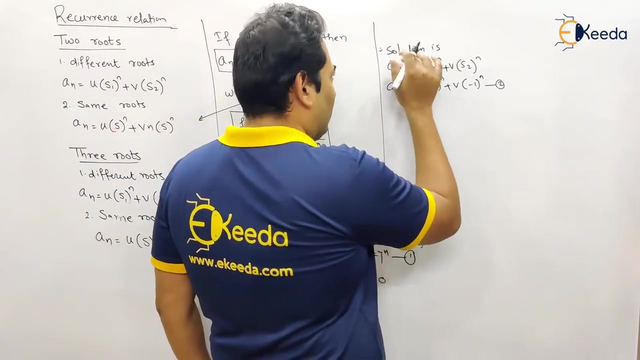 since there are two roots, your solution is a. n is equal to this, but in that case if we have f of n- see here- we have f of n- then the solution becomes a n h plus a n p. so in that case, this solution is not the final solution. this solution is a n. 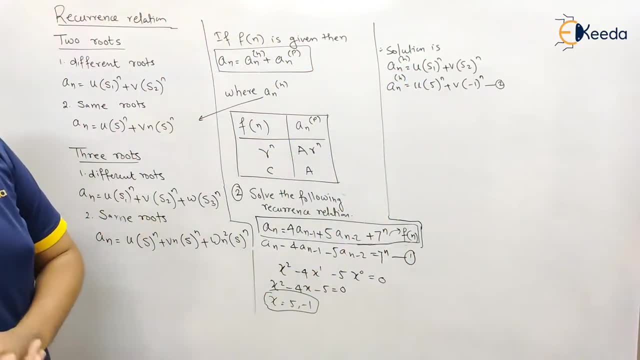 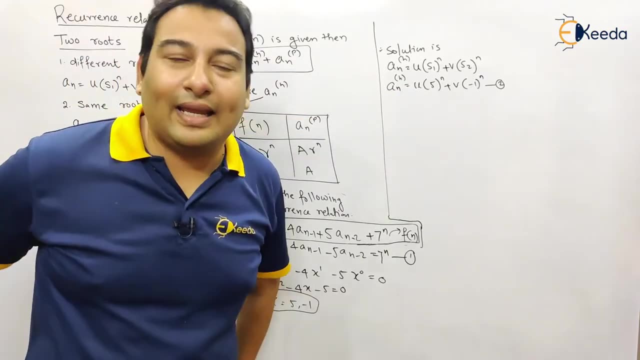 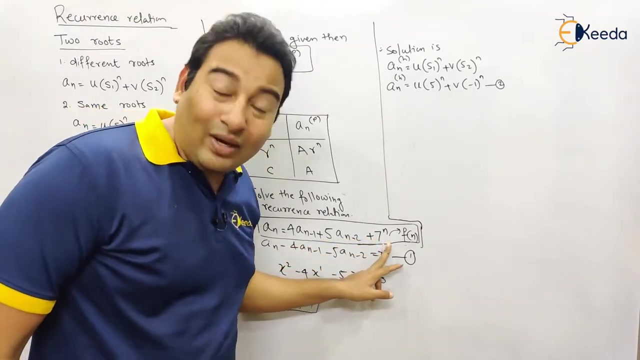 h. it's not final solution. final solution will be a n h plus a n p. if this is not given, this is my final solution. that is your a of n. now we need to find it out. a n p, suppose, along with that 7 raised to n, along with. 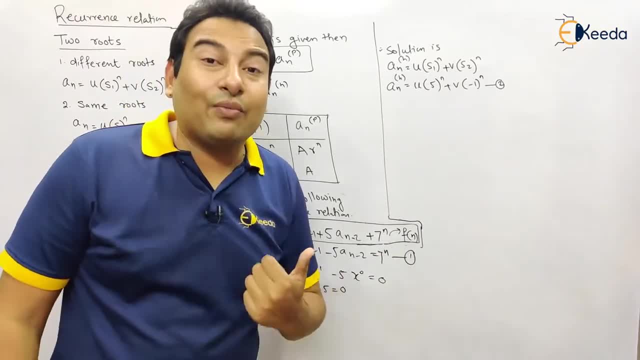 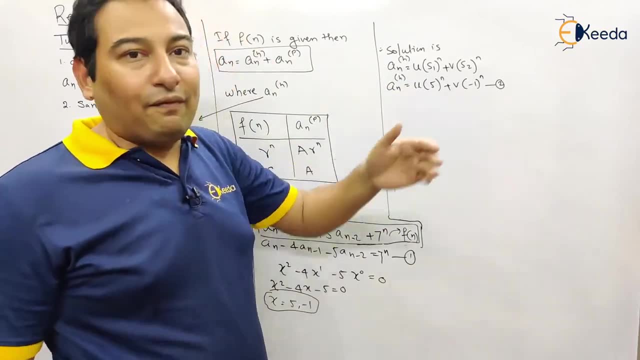 that initial conditions are also given. that likewise given in the first problem, then will not stop here for a, n, h, we will go ahead and we will find the value of u and v that we did in the last problem. let us move on now. we will find it out. a. 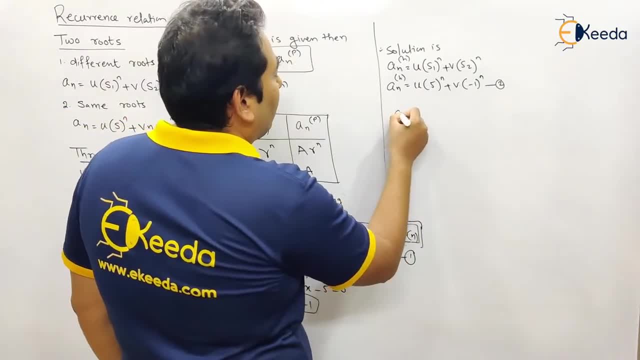 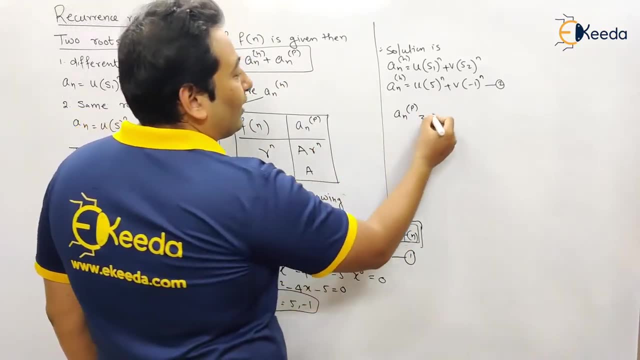 n p. so here a n p is a n p depends upon your function. here it is r raised to n, so a n p is a r raised to n. so a is from our side and r raised to n will remain as it is. so r raised to n means. 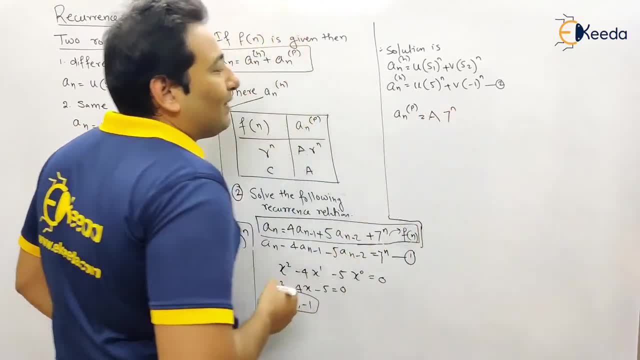 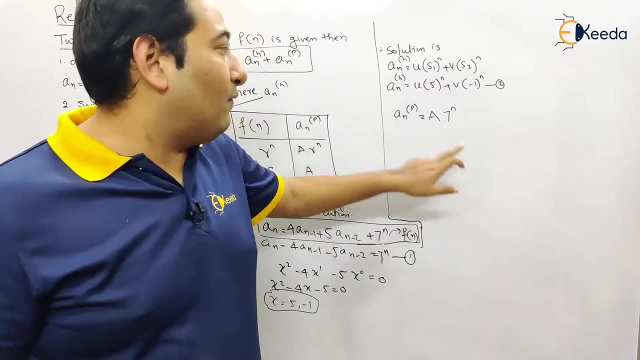 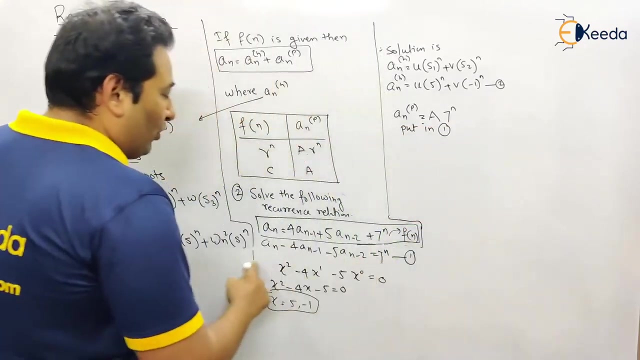 the function, that is 7, raised to n. so this is my a n p. in a n p i want to get the value of a. so see the procedure, what we'll do to get the value of a. we're going to put in equation number one. let's put in equation number one. see the procedure we're going to substitute in equation. 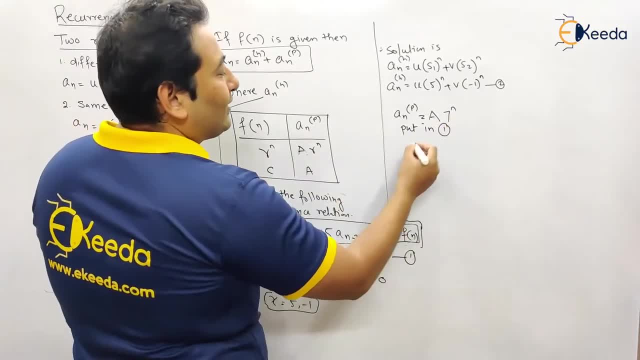 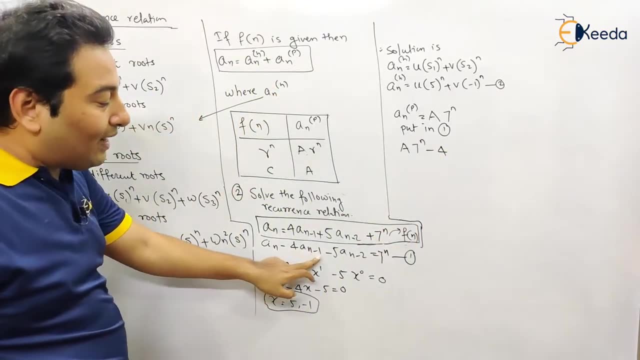 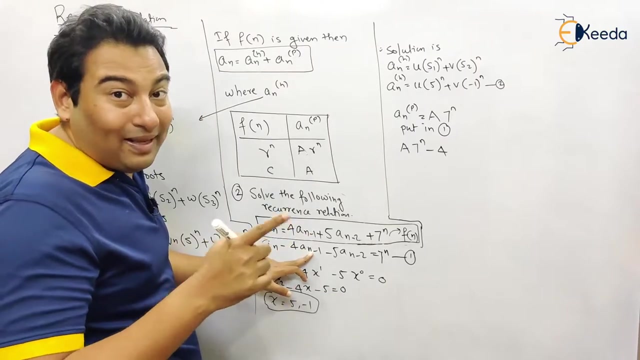 number one. so in place of a? n, we're going to put a seven days to n. what else minus four? see this minus four. a of n minus one. a n is a seven days to n, but here it is n minus one. that means we need to replace n with n minus one, so this will become a seven days to n minus one. 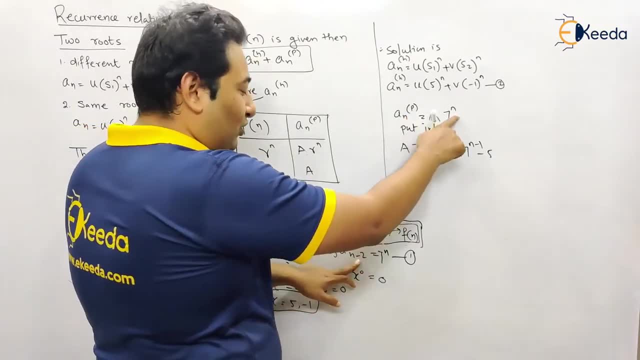 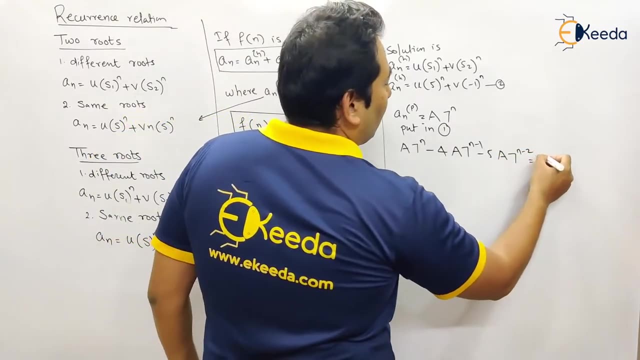 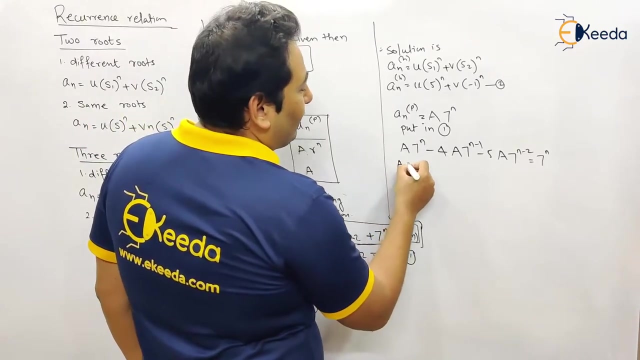 minus five, a n minus two. so a n is a seven days to n. here it is n minus two. so it will be a seven days to n minus two, equal to right hand side seven days to n. we're going to put in equation number one, so this is a seven days to n minus four, a seven days to n upon seven, obviously seven days. 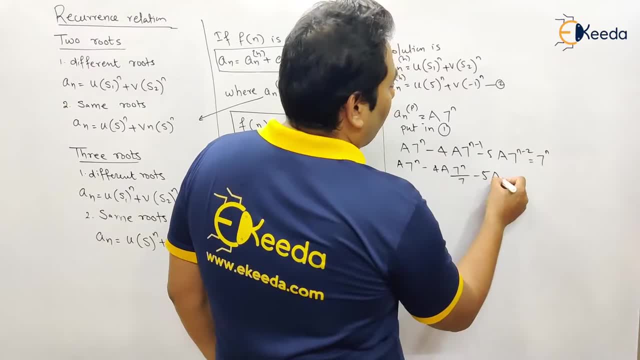 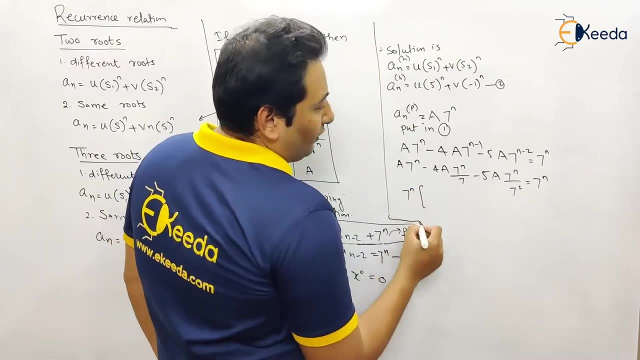 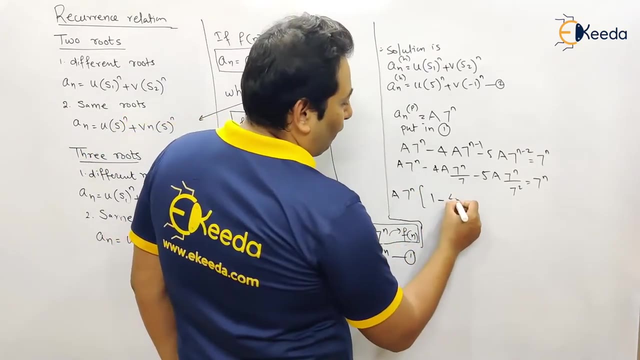 to n minus one can be written in this format: seven days to n upon seven square you let's take seven days to n common inside, or we can take a seven days to n common. so here it is one minus four by seven, because we took a seven days to n common, so we left with four by seven. 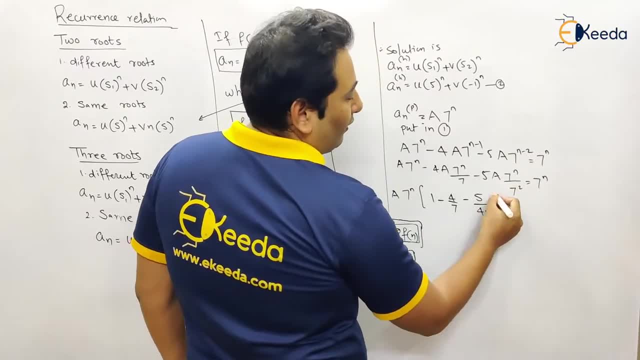 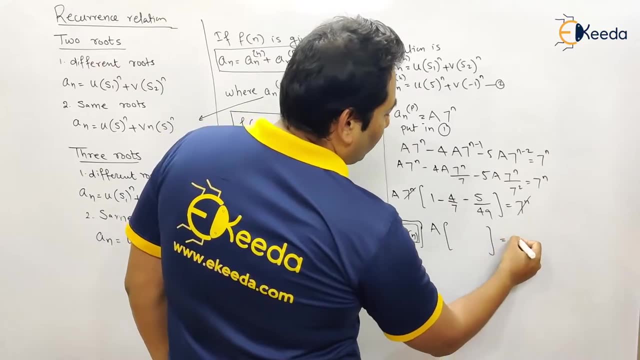 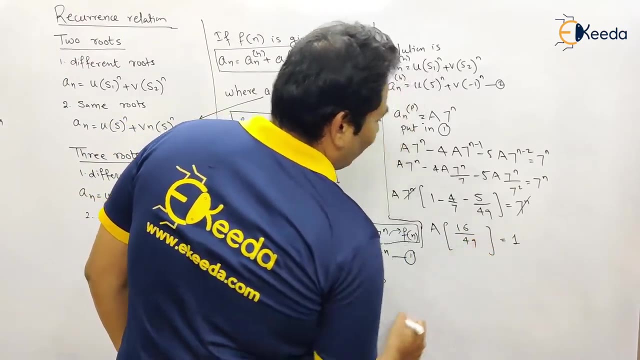 minus five upon forty. nine is equal to seven days to n, so that will be cancelled from both the sides. a in bracket. we need to solve this, so let us do the calculation. sixteen by forty-nine. therefore, a will be equal to this, forty-nine will go up and sixteen will go. 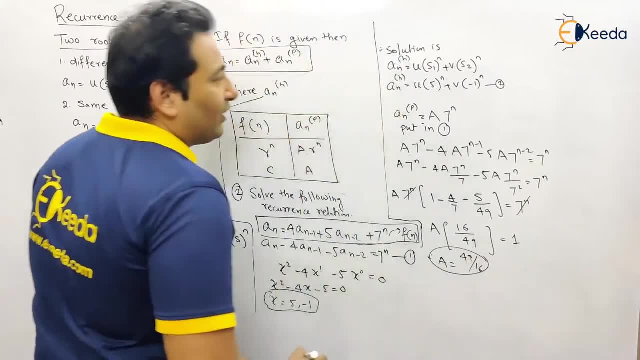 down. so that is forty-nine multiplied sixteen. so this is a. we got a and p. let us put in equation number three. if you do that, we'll get the value of a and p, that is forty-nine multiplied sixteen, into seven days to n, and that will give us: 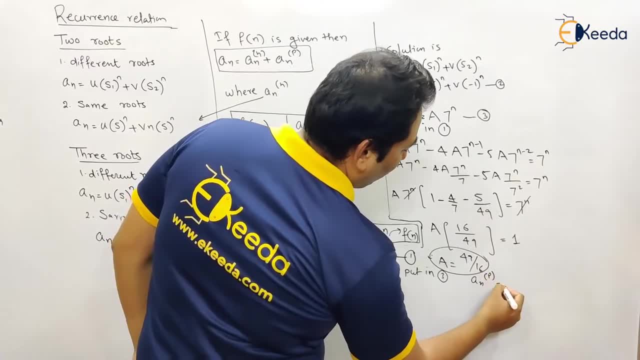 Mistakenly dangled, comfortable work. fossilوبility test- proper test. are you trying this test all these eight days and any hundred days before to? if you give us a less than answer, because we're still here- life and water series now, this is adding value much less than it is road里ferhhardt, and we'll go to another.